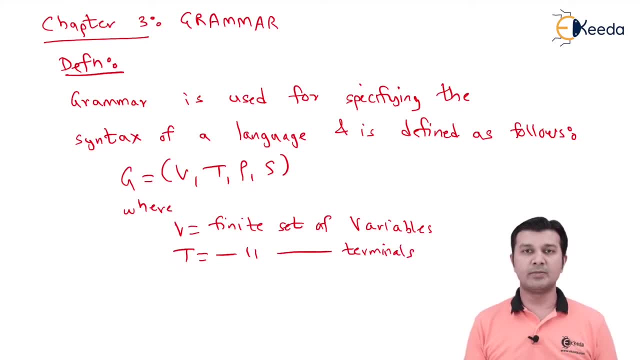 Now what I mean by terminals. exactly opposite to variables. if variables are capital alphabets, terminals are going to be small case alphabets. The next is I have p. p is called as the finite set of production rules. So p is the finite set of production rules And lastly, s is called as the 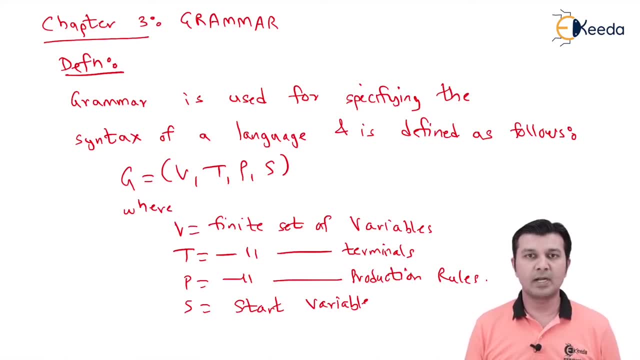 start variable. So that's how we define the grammar. g is equal to v, t, p, s, where v is nothing but capital alphabets, My t is nothing but small alphabets. We are going to be some production rules which is going to be used for deriving the grammar. Of course, that is going to be the heart of the grammar. That is the one which is actually going to help us derive anything, And s will be called as the start variable. Moving to the next definition, 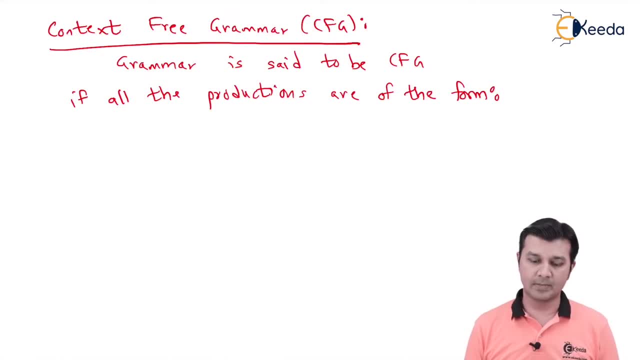 So here we have context free grammar. So I define a context free grammar as a grammar is said to be cfg if all the productions are of the form a derives alpha. Now, what I mean by that? I mean to say that when I say a derives alpha, a is going to be called as a capital alphabet, Remember which we called as a variable. 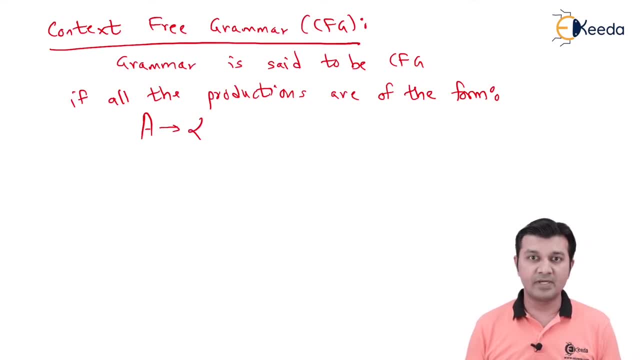 So a is equal to v, t, p, s, And over here a is nothing but that v. So a is a variable and alpha is anything which is in sentential form. Therefore I say grammar is said to be cfg if all the productions are of the form. a gives alpha where my a is a variable and alpha is in some. 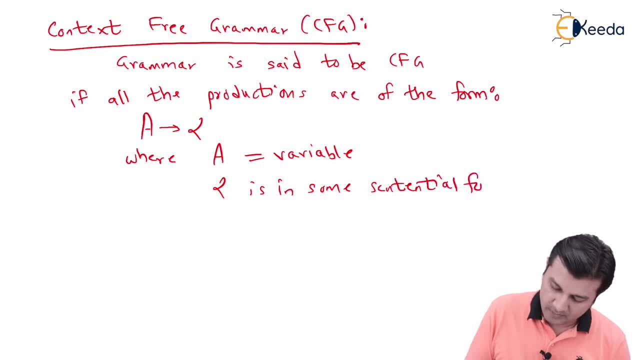 sentential form. Now, what I mean by sentential form? it should be able to derive some sentence. Let us take an example. So the example over here says I have my production rules, something like this: Let us say my p is called as the production rule and the production rule is s gives a, s, b. 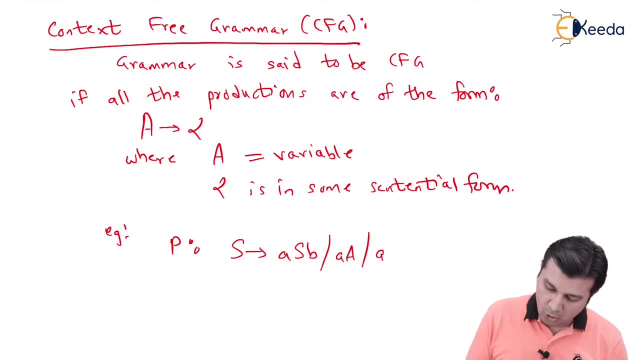 Or s gives a a or s gives simply a small a. Similarly next, I have a gives a capital, a small b, or a gives b. Now, if I look at this problem, let us try to understand what do I exactly mean by this. So I say over here that my s is capable of deriving a s b Right. 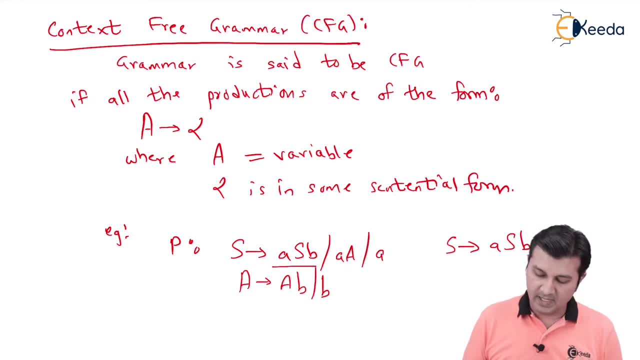 Now, how is that possible Using this production rule s est b? Further, if I look at the next capital alphabet- remember a golden rule: the movement- I get small alphabets. it is the end of it, because everything in small alphabet will be called as a string, Whereas if the string contains any capital alphabet, that is variables. 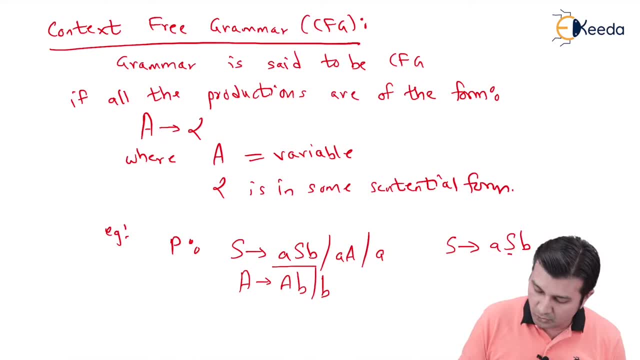 I can further derive it. So if I see you over here in arrow ASB, that s can further derive me something, now that something can be anything among ASB or small a capital A or small a. so let's say this time I say that my center s has given me small a capital A and rest everything before and 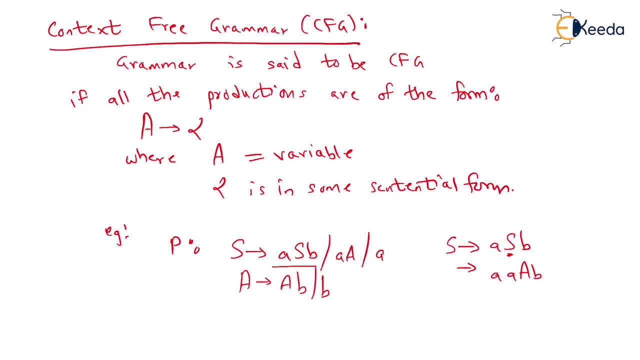 after it remains the same. so now the string which I have, or rather I would say an incomplete string, a small, a small a capital, a small b. now my capital a can further derive something, and for a also, I have a total of two combinations. so let us say, among these two combinations, my a selecting this combination b1. so I 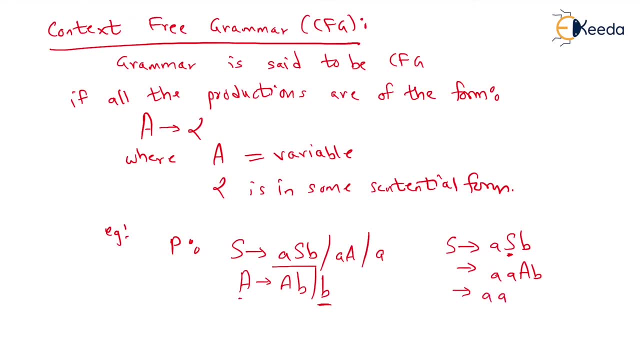 say a gives simply a small b and small b remains over here. so can I say overall that my grammar b, A and small b. so I say small a and small b are the terminals. what are the production rules, the one which we? what are the production rules, the one which